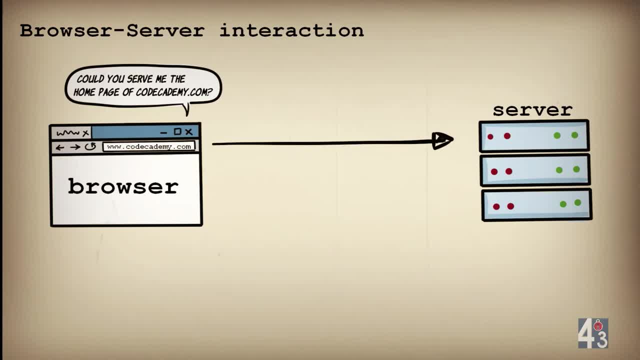 bar and press enter, you are essentially requesting a server of the corresponding website to deliver the website's homepage to your browser. Now, this interaction that you have with the server via your browser is called a request. The same applies when you click on links on the website, Let's say you click the login. 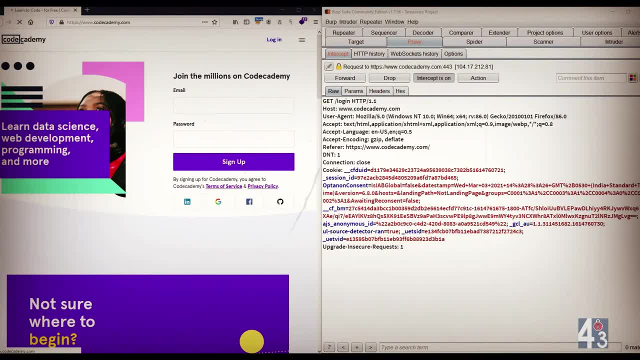 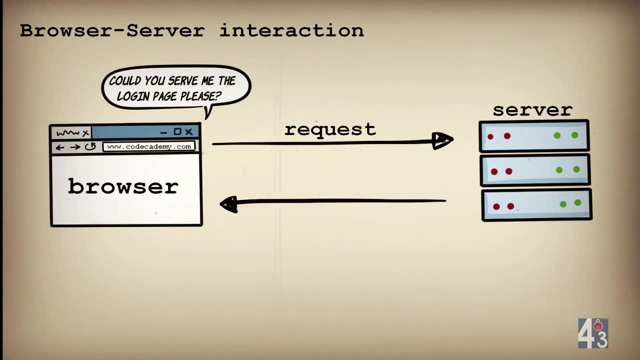 option. You are requesting the server to serve you the website's login page. So this is what the request would look like. Note that the request asks the server to get the login page of the website. This is called a get request, Correspondingly the act of the server delivering the login page of the website to your browser. 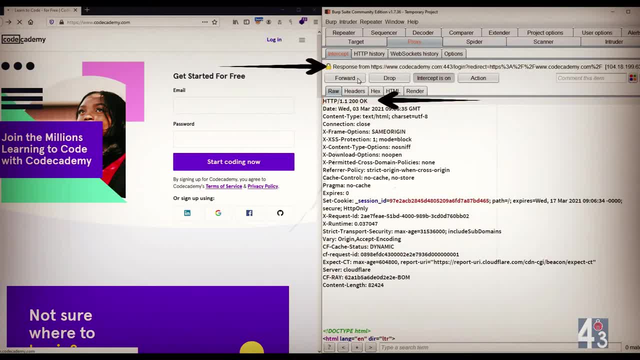 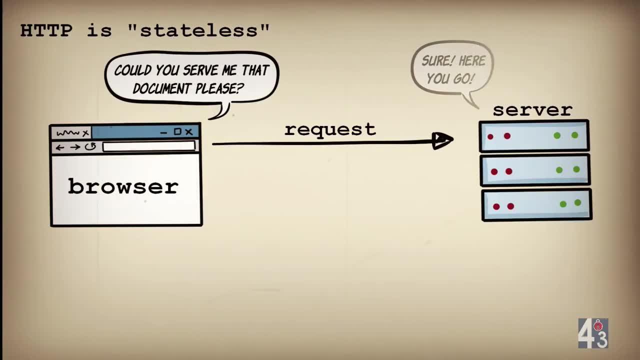 is called a response. Note that the server responds with an OK and delivers the login page. The internet and HTTP were initially created to share documents. That's all there was to the internet. They were not designed to operate the way it does today. There was no need for. 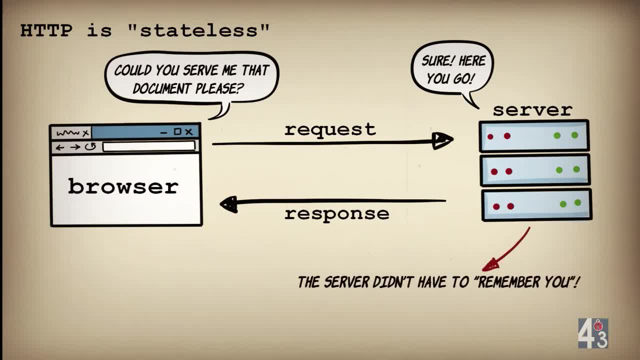 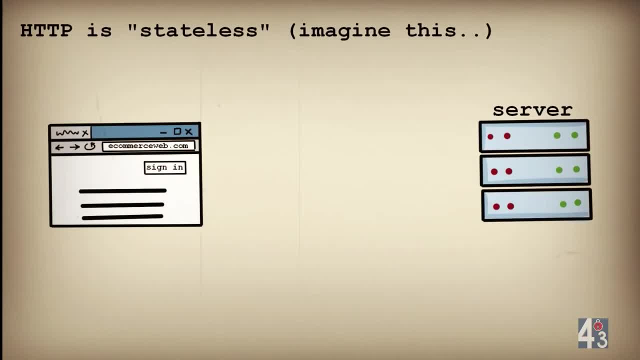 the server to know or remember who you are. Now, if HTTP were to be used like this today, applications would make our internet lives frustrating. So imagine this: You click, sign in on, let's say, an imaginary website called ecommercewebcom. 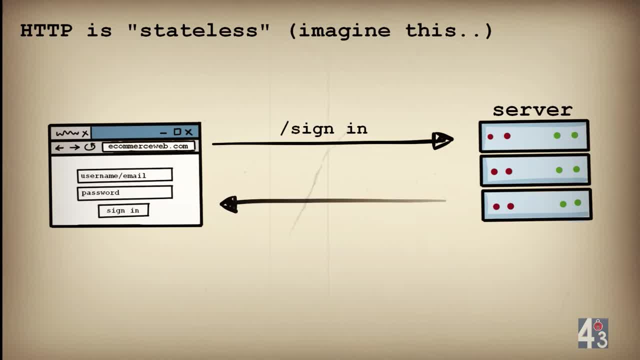 via your browser. Now ecommercewebcom's server responds with a sign in page. You type in your credentials and click sign in. ecommercewebcom's server responds with a home page. So you click on the orders option to check your order history, But ecommercewebcom's server responds with: 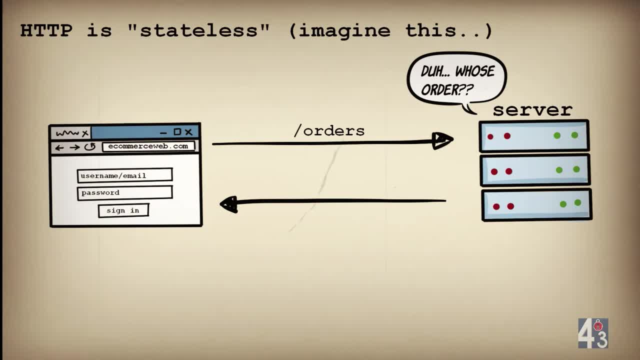 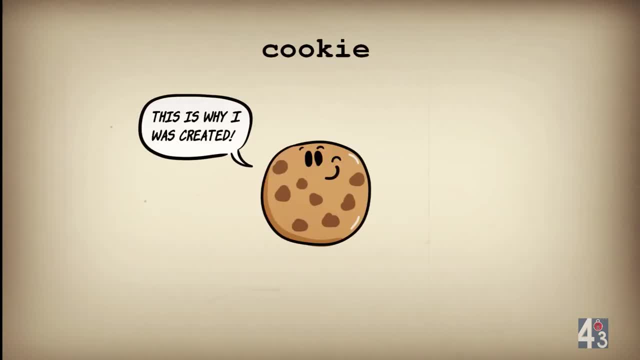 a sign in page. You see, the server is unable to remember who you are. For every personalized request you make, it would ask for your credentials. So this is why cookies were created in the first place. This is how set websites remember you and your preferences. In technical terms, cookies- 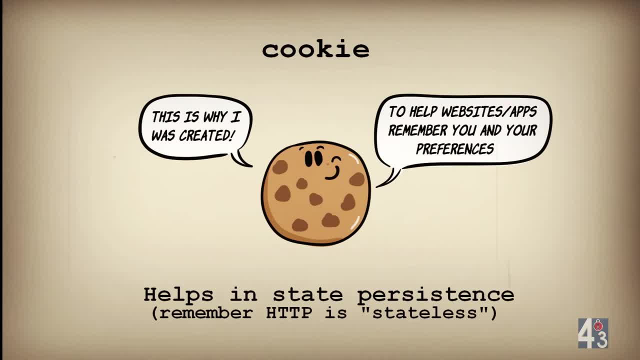 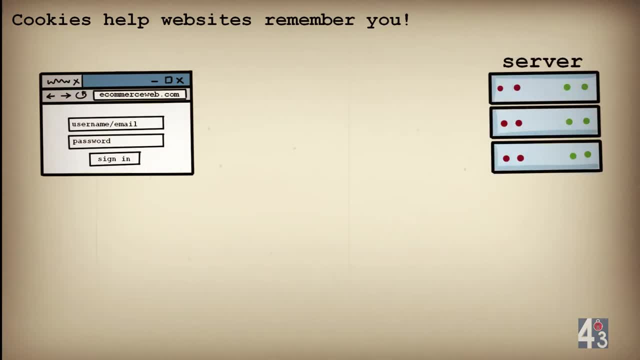 help in state persistence. So how does this work? So let's imagine John is signing in to ecommercewebcom for the first time. John types in his credentials and clicks sign in. ecommercewebcom's server responds with a home page. Now note that the 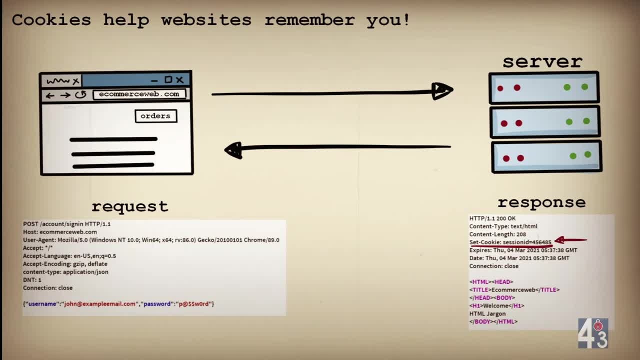 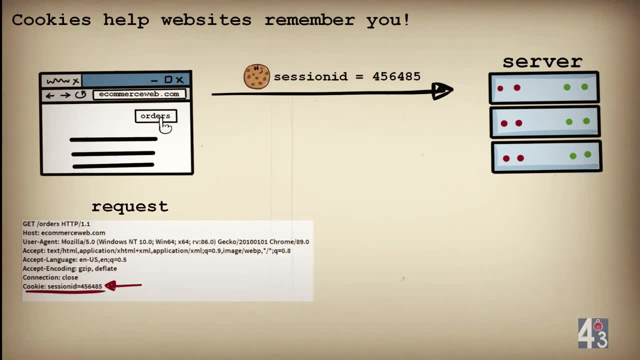 server adds a set cookie header. The server is assigning John a cookie by the name sessionid and value 45645.. John clicks on the orders option to check his order history. Now note the cookie header in the request. Once a cookie is set by the server in the first response, the browser. 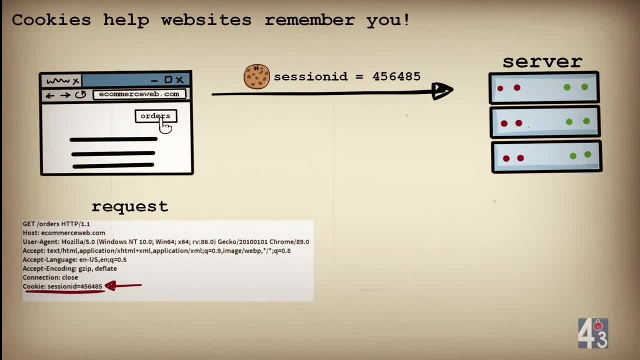 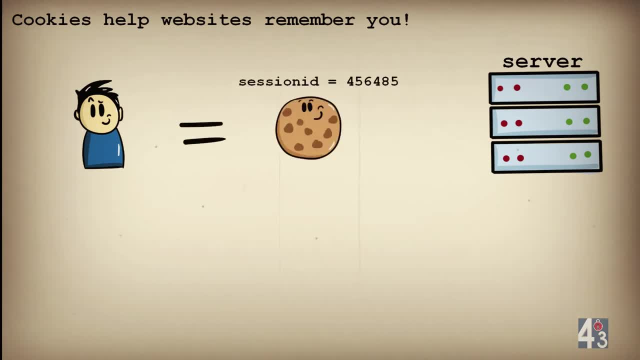 will add the cookie header with the name and value in every subsequent request John makes. So this cookie sessionid456485- assigned to John is an identification. The server will now remember John as sessionid456485 on every subsequent request. This is because the server sets a file in its disk corresponding to the cookie set for John. 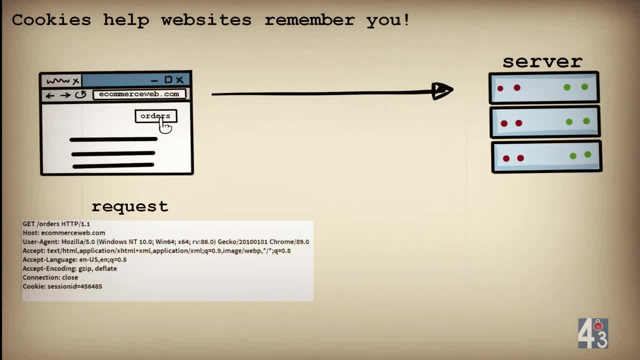 So when John clicks the orders link after signing in, the server checks for the file corresponding to the cookie it received from John's browser, recognizes it is John and responds with John's order history page. So this is how a state is persisted. 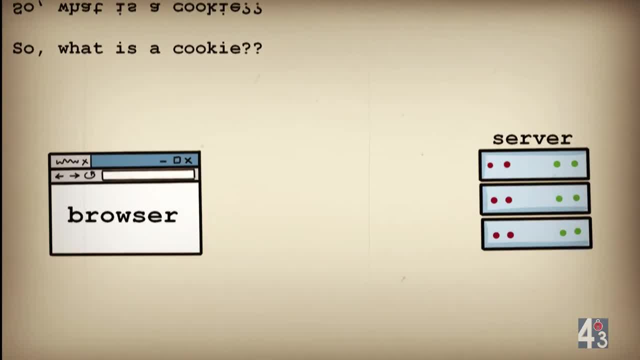 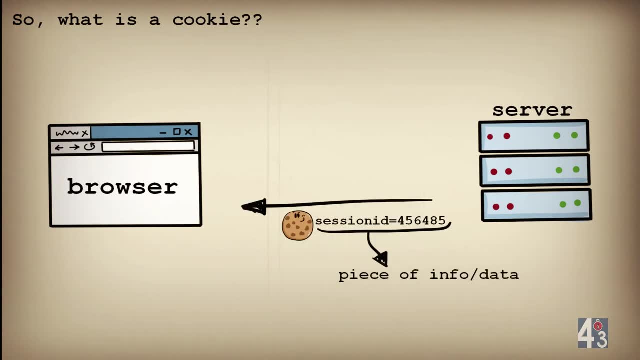 This is how ecommercewebcom remembers John, So defining what a cookie is would make more sense now. So cookies are basically small pieces of information or data that a website or web server sends to your browser via the set cookie header so it can be stored in your computer's hard disk. 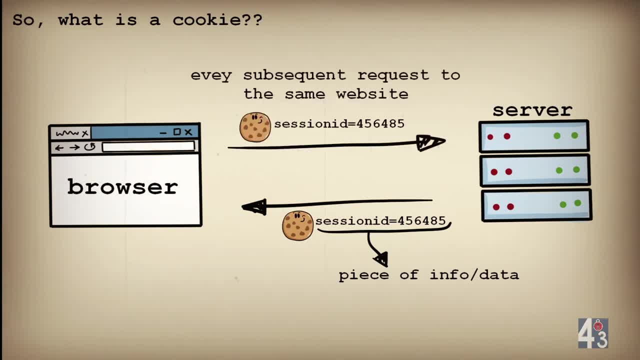 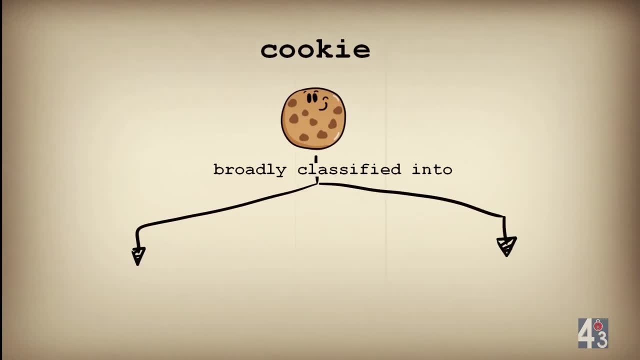 And the next time you make a request on the same website, your browser sends the cookie via the cookie header along with the request, so the website can identify you. Cookies can be broadly classified as first-party and third-party cookies In the previous example. 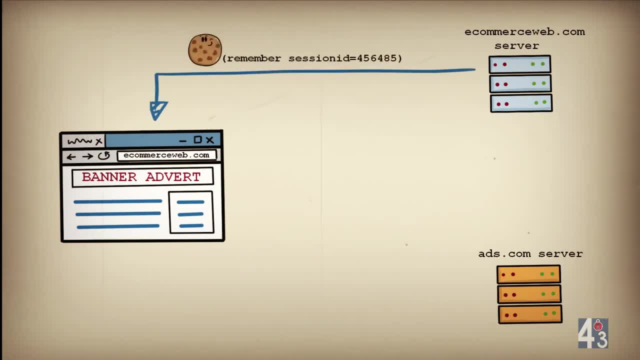 session ID 456485 was set by ecommercewebcom for John. This is a cookie set by the same website John is currently or directly browsing. Hence it is called a first-party cookie. But what if ecommercewebcom had ads on their webpage? 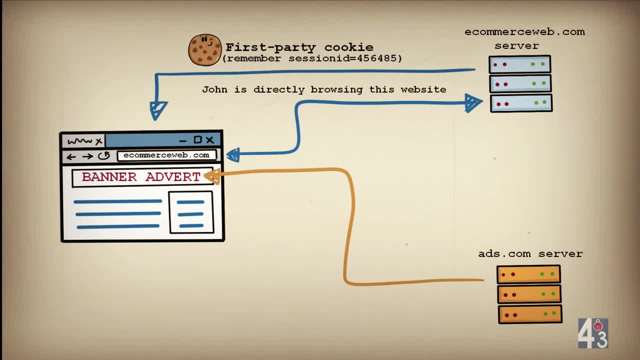 These ads, though, seen on ecommercewebcom, are being served through another server, let's say adscom. So when John visits ecommercewebcom for the first time, the adscom server serving the banner ad could set a cookie header for John. 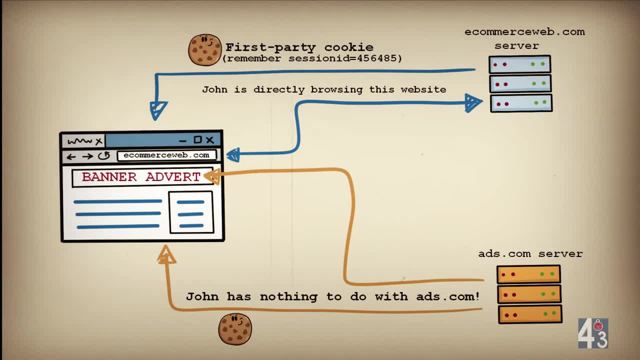 Now, this is a cookie set by another website. John is now directly browsing. He's on ecommercewebcom. The cookie set by the ads server is a third-party cookie. While there are many different ways companies use to track you online, third-party cookies are an important tool with which they can achieve the same. 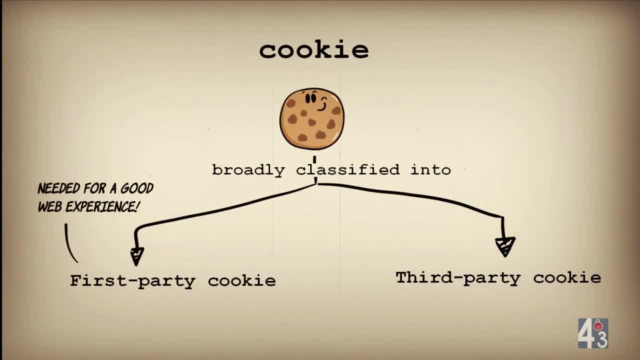 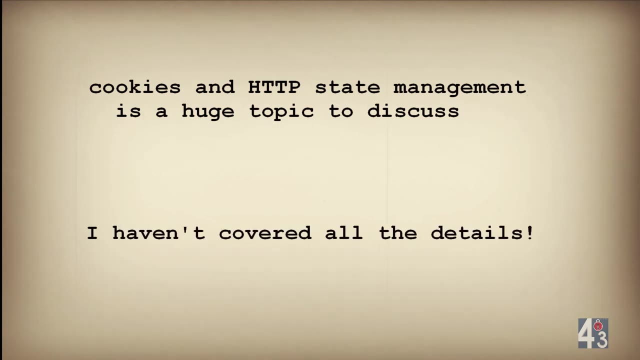 Remember, first-party cookies are needed for the web to function well, whereas user tracking for targeted ad-serving purposes is achieved with third-party cookies. Cookies and HTTP state management is a huge topic to discuss and I have not covered everything related to this topic.